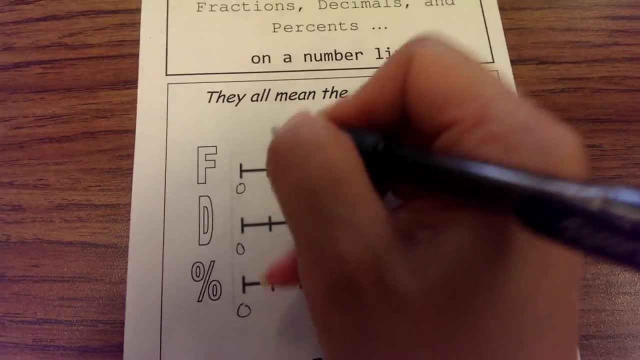 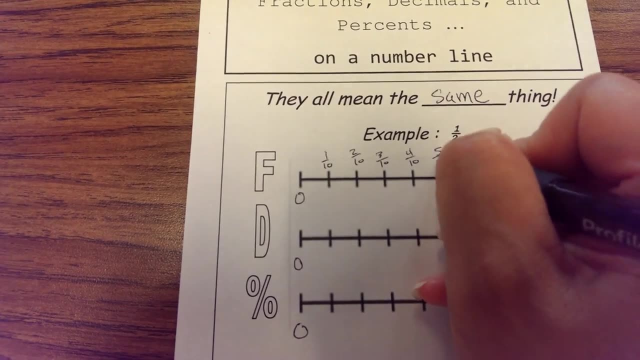 Therefore, each tally must be worth 1 tenth. So this would be: 1 tenth, 2 tenths, 3 tenths, 4 tenths, 5 tenths, 6 tenths, 7 tenths, 8 tenths, 9 tenths. 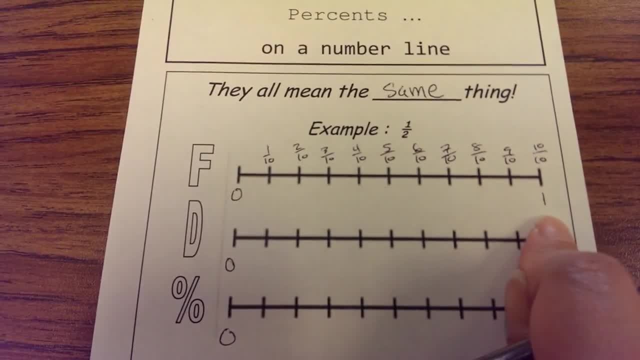 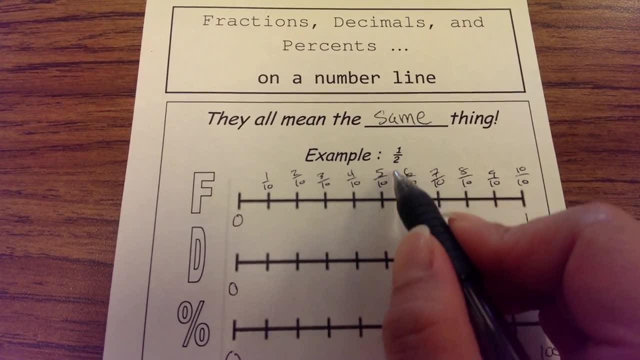 and, of course, 10 out of 10 would equal a whole. But then where's a half? Well, 5 tenths is the same thing as a half. If we simplified 5 tenths, it would simplify to a half. 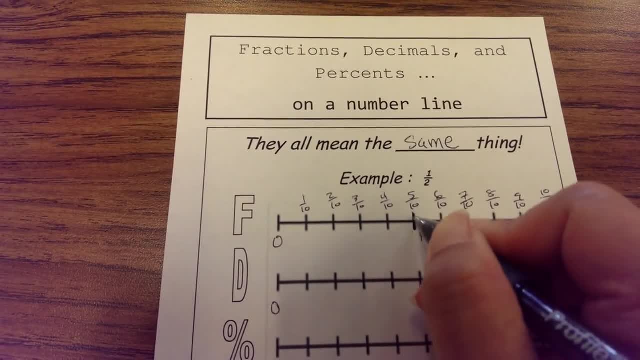 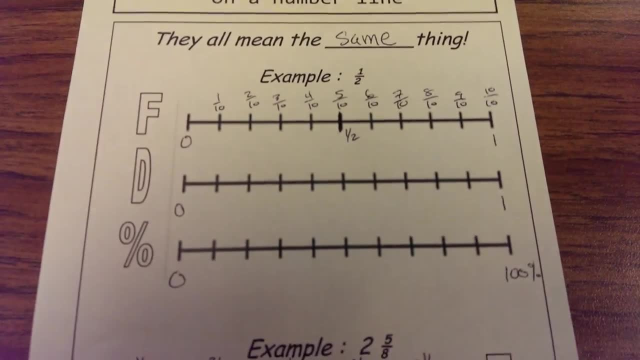 So here is our halfway mark. This would be a half right there. Start This dark tally right there. That would be where the halfway mark would be. Well, what if we were talking about decimals? The 0 starts here. The 1 starts here. 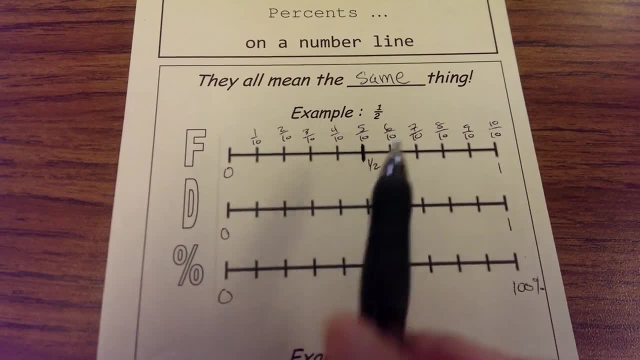 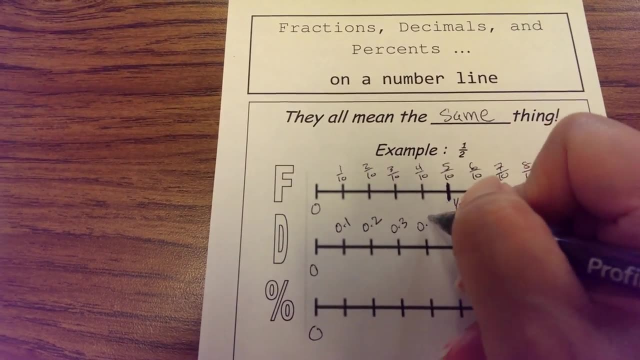 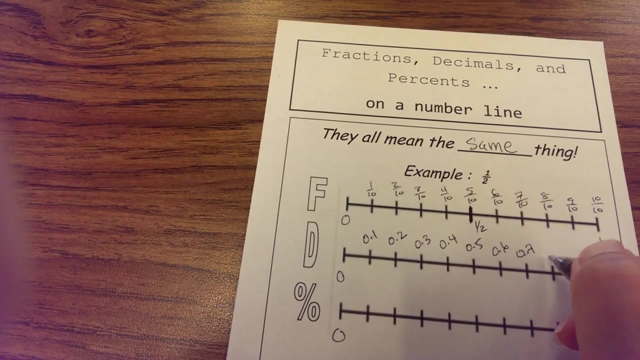 Each tally would be a tenth and we can change each of these tenths into decimals: 1 tenth as a decimal would be 0.1.. 2 tenths, 3 tenths, 4 tenths, 5 tenths, 6 tenths, 7 tenths, 8 tenths, 9 tenths and then 10 tenths would be a whole. 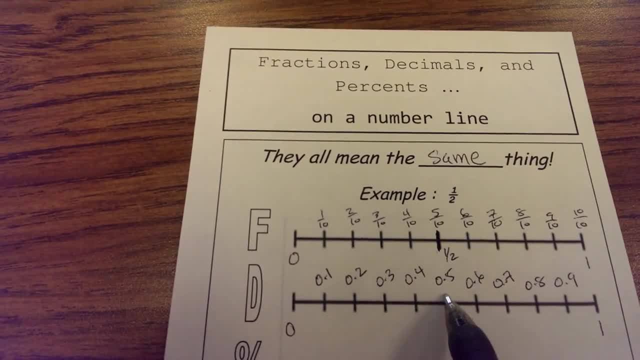 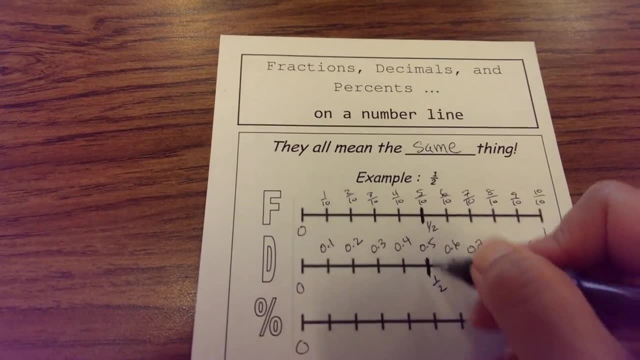 Again, where would the half be? Well, a half written as a decimal is 0.5.. So this would be where the halfway mark would be. So you can see that it matches with the fraction number line. Last one as a percent. 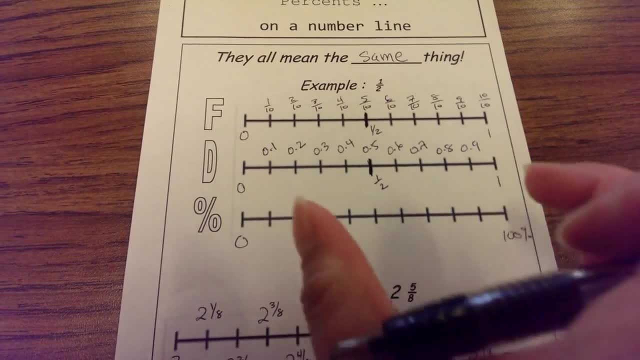 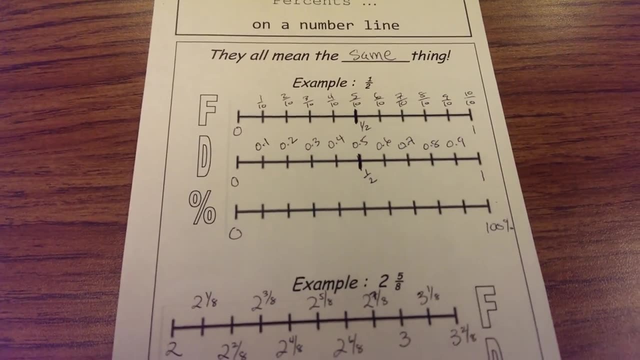 Well, as a percent, the 1 whole would equal 100%. If you got a whole candy bar, you got 100%. So the 1 whole, the 100% would be where the 1 whole is Half. well, what's the percent for half? 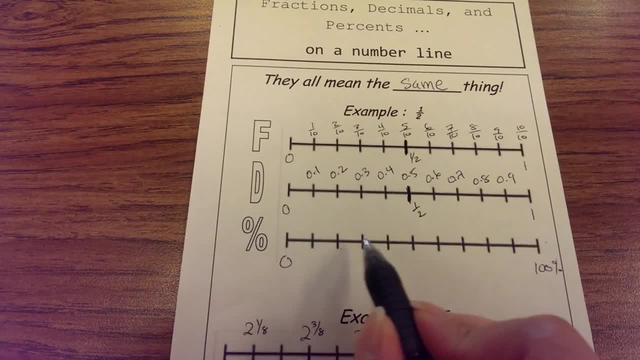 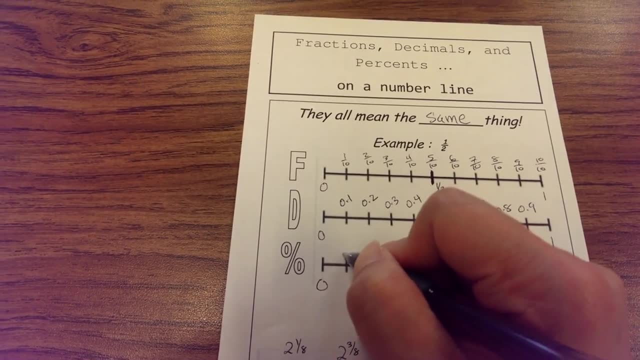 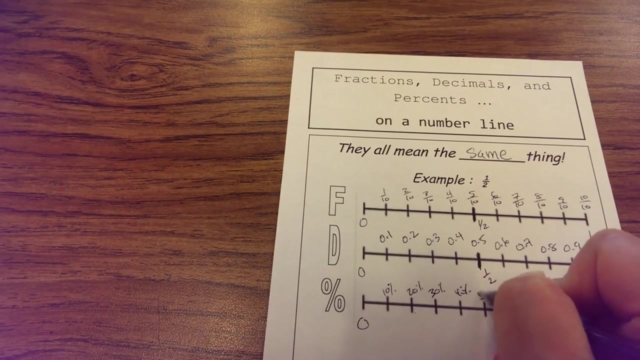 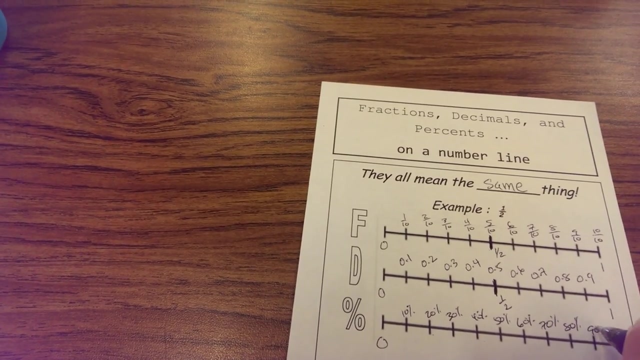 The percent for half would be 50%. So then this: each of these. again, there are 10 tallies. So if I need to get to 50%, each of these would be worth 10%. So then this is 10%, 20%, 30%, 40%, 50%, 60%, 70%, 80%, and this would be 90%, and then we would get to 100%. 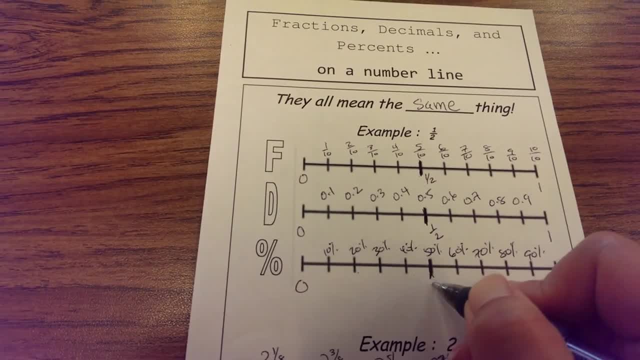 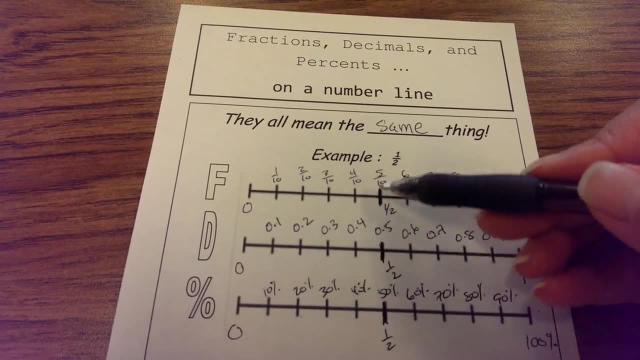 And a half is equal to 50%, So that is where the half would be on a percent number line. So you can see that they all mean the same amount, Just three different ways of representing them. Let's look at this next example. 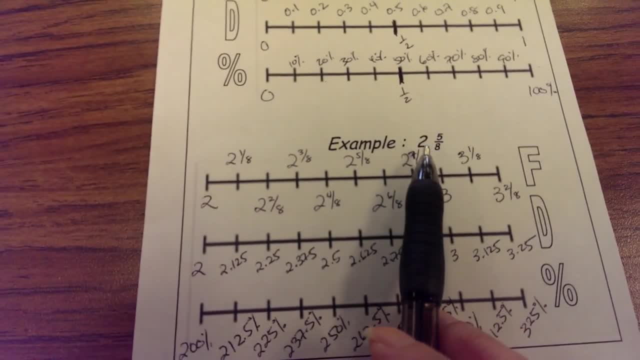 We've got 2 and 5 eighths. So, based off of my number line, since I need between 2 and 3, I did my number line between 2 and 3 over here. Now the 3 is not the end. 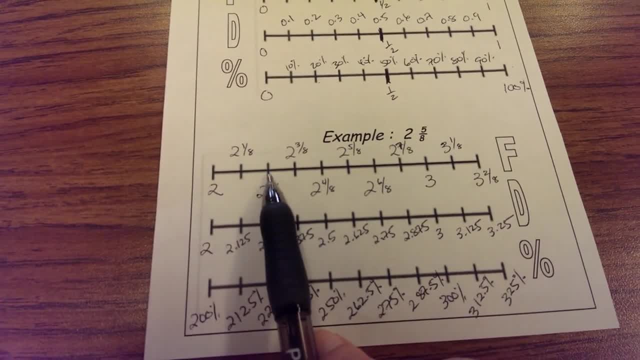 Why? Because it goes by eighths. So I said each of these tallies is an eighth. So that's 1 eighth, 2 eighths, 3 eighths, 4 eighths, 5 eighths. 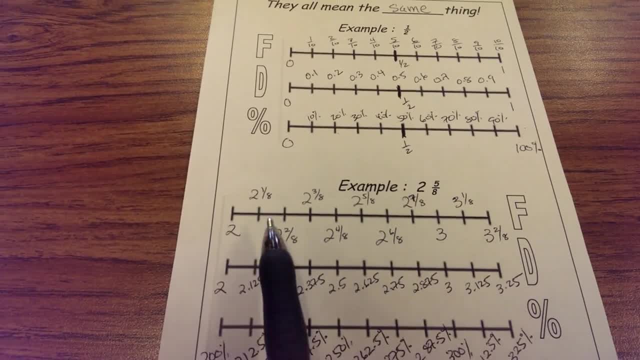 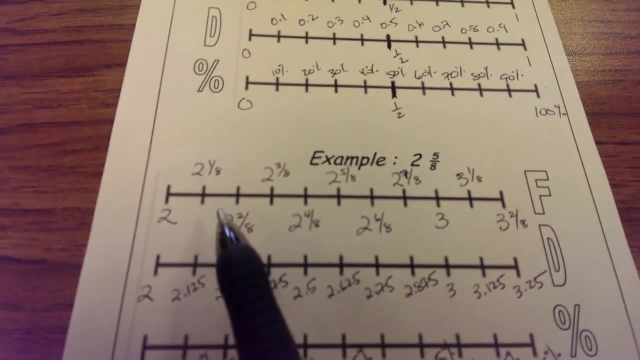 6 eighths, 7 eighths, 8 out of 8 would give you another whole right. So my 3 does not go in here, because each of these were worth an eighth. So now that I've numbered it as a fraction- 2 and 5 eighths- well, here's two wholes. 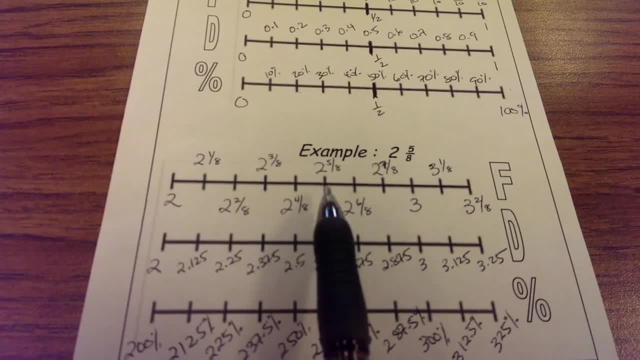 Here's 2 and 1 eighth, 2 and 2 eighths, 2 and 3 eighths, 2 and 4 eighths. There's my 2 and 5 eighths, So this is where 2 and 5 eighths would be. 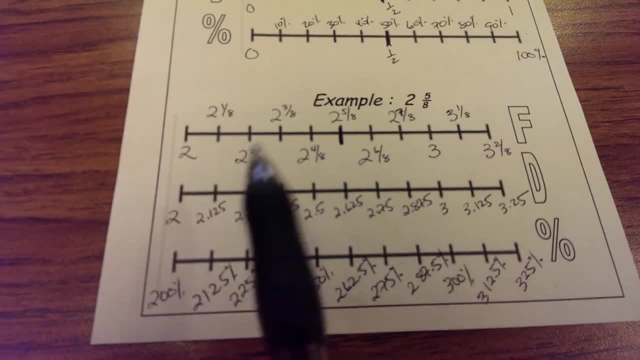 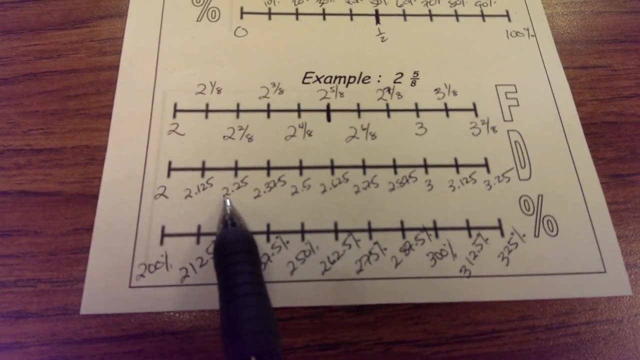 Well, what if I changed the number line to decimals? Well, if it were decimals, instead of writing 2 and 1 eighth, I would write 2 and 125 thousandths. This would be 2 and 25 hundredths. 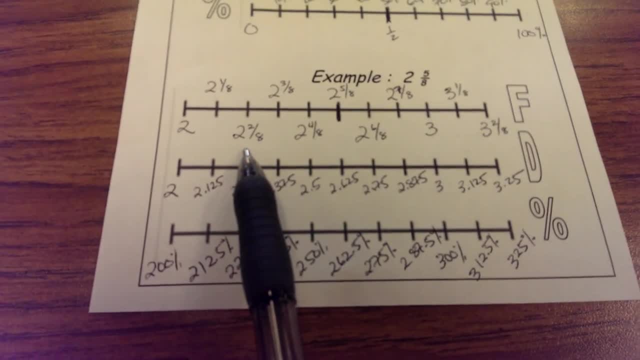 Same thing as 2 eighths. 2 and 25 hundredths is the same thing as 2 and 2 eighths. So I wrote all of these, I changed all the fractions into decimals, And where would 2 and 5 eighths be? 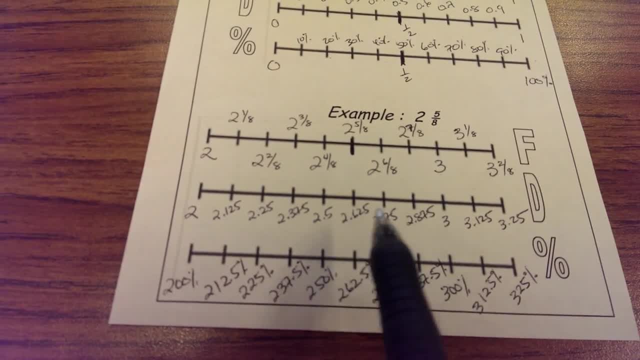 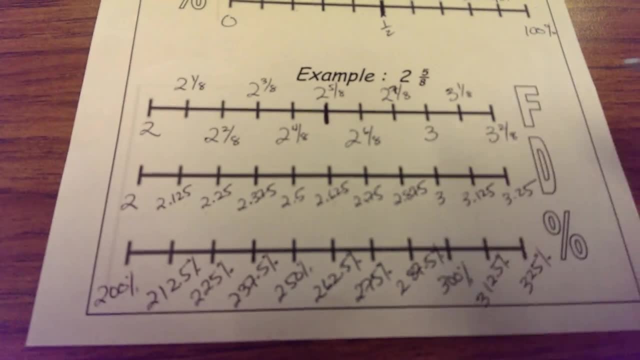 Well, 2 and 5 eighths as a decimal is 2.625.. 2 and 625 thousandths, And you can see it would be right there, right, So 2 and 5 eighths and 2 and 625 thousandths means the same thing. 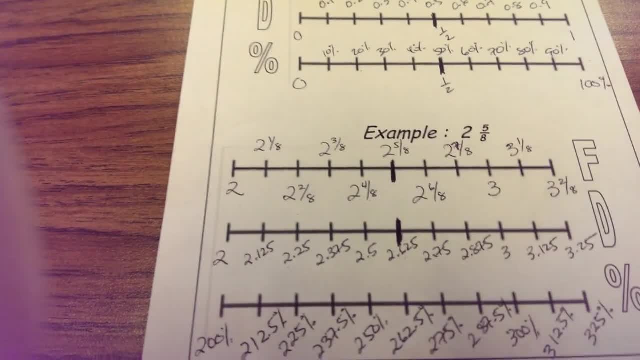 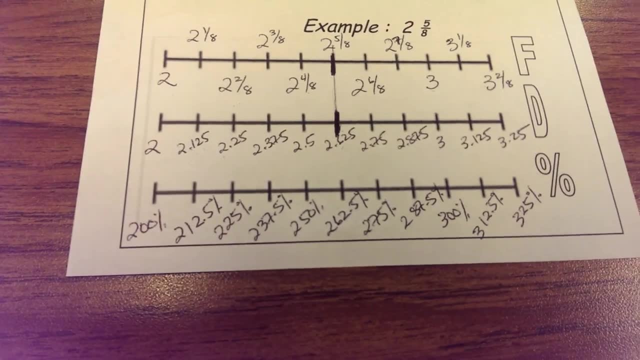 So that is also where it would be. I'm going to do a little dotted line so you can see it, And then if I change it to percents, well it's going to be. these percents are really high Because, remember, if you have one whole, you have 100%. 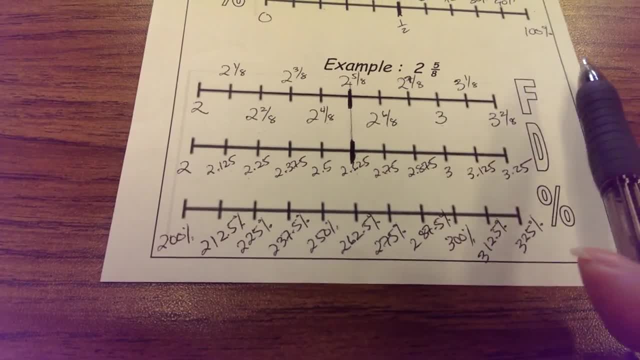 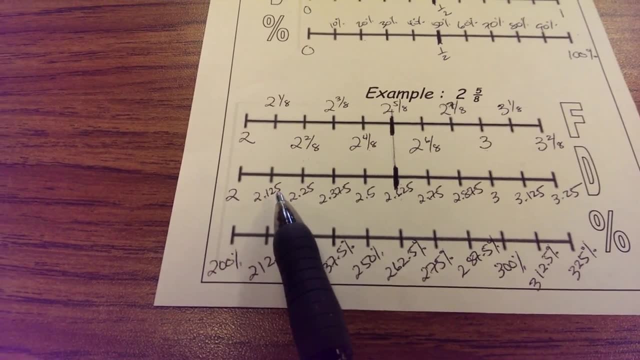 We have two wholes and then 5 eighths of a whole, So it's going to be over 100%. The two wholes would be 200%, And then I changed each of these into percents. All I did was move the decimal two spaces to change the decimal to percents. 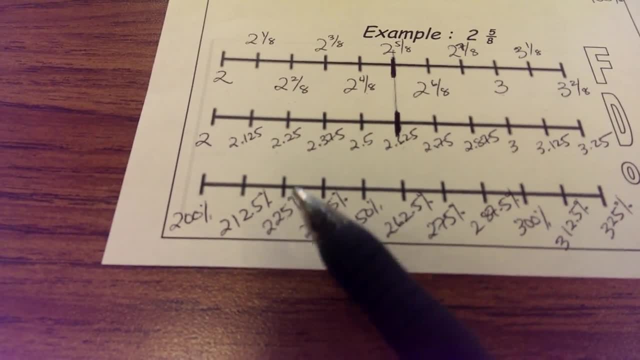 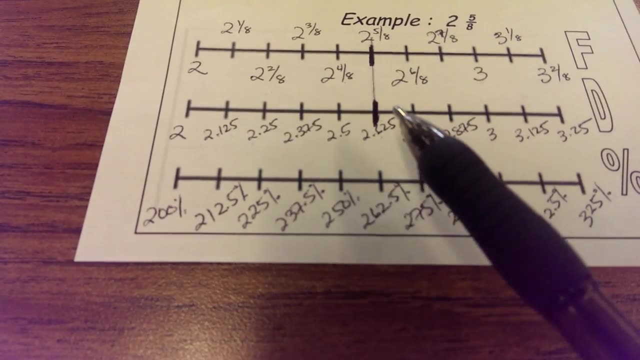 So you can see, I've got 212.5%, 225%, 237.5, and so forth, Until I get to 300%, which is where the three wholes is. Well, what is 2 and 5 eighths as a percent? 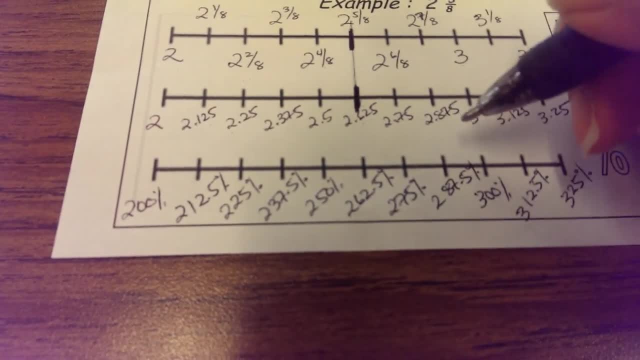 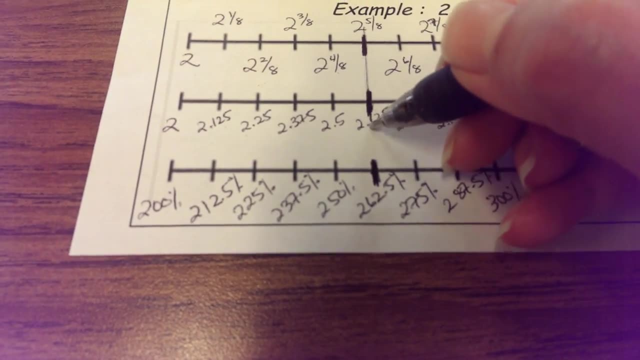 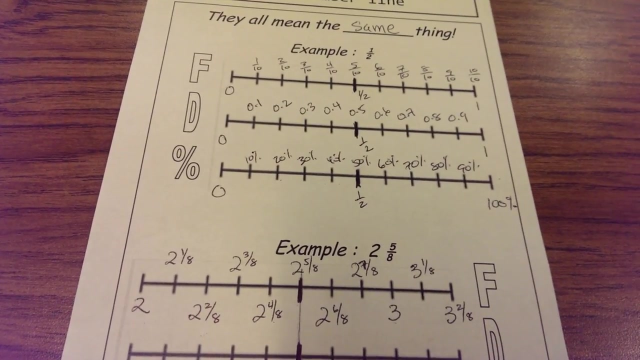 It would be 262.5%. So this is where 2 and 5 eighths would be on my percent number line And, as you can see, it matches up. It matches up with the other two And this is how we represent fractions, decimals and percents on a number line. 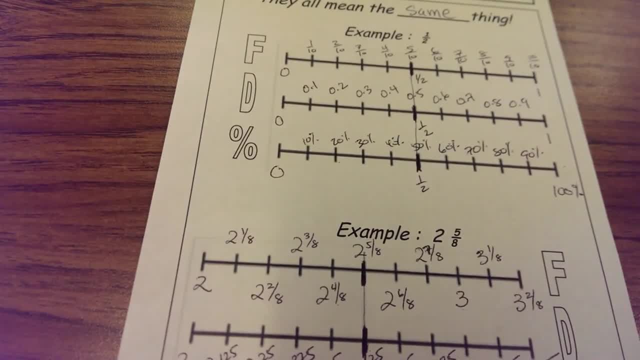 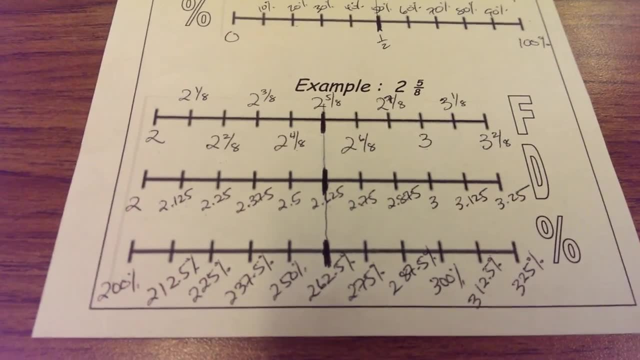 They all end up being the same. The halfway mark is the same there, And then the 2 and 5 eighths. whether it's a fraction number line, a decimal number line or a percent number line, it ended up being in the same spot. Because it means it's the same value. 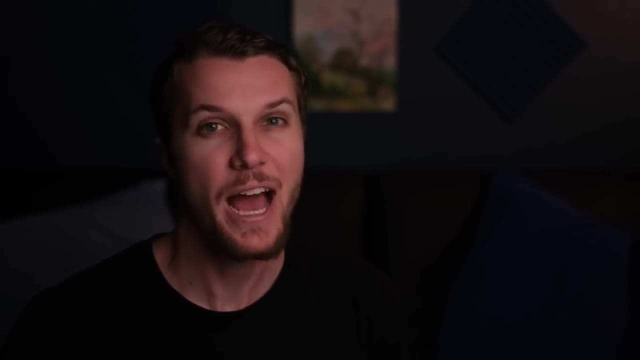 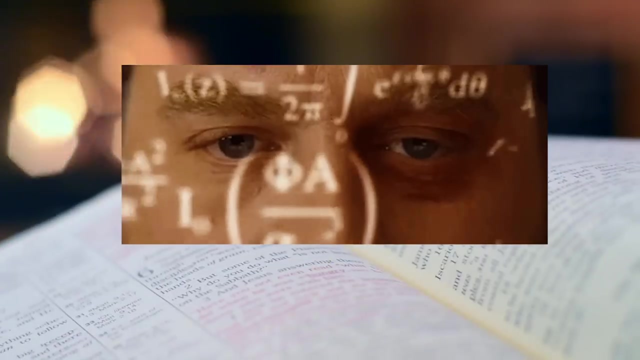 Without data structures you can't solve algorithms, And without algorithms you can't pass a programming interview. Now the problem is: if you open a data structures and algorithms textbook, it is really mathy. And if you're like me and you got a C in eighth grade, 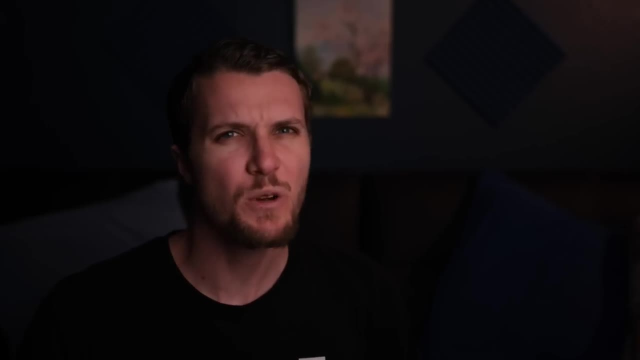 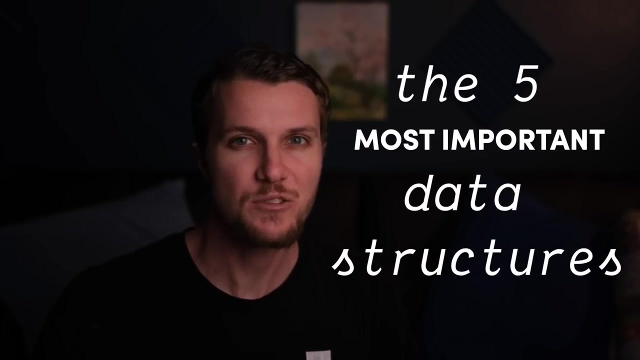 math. it's going to scare you a lot. The good news is, once you understand data structures, they're not actually that complicated. So I wanted to explain the five most important data structures in this video in the way I understand them, which means as little technical. 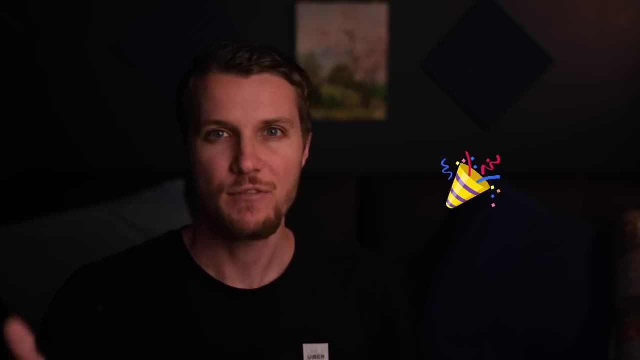 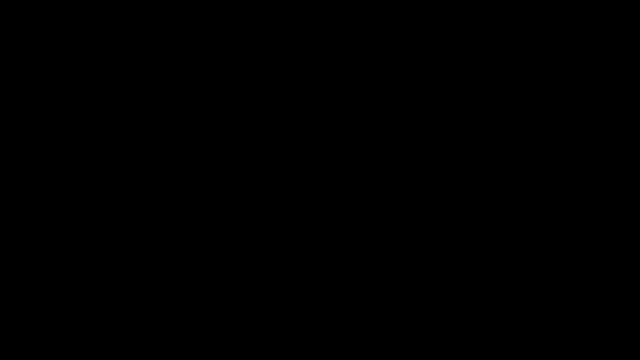 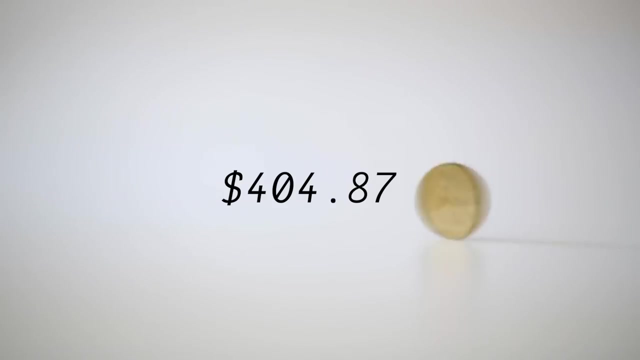 jargon as possible and just try to simplify it for you guys. just starting out, Let's go First off. let's talk about what a data structure is. Consider having a single data item like the price of a stock. Now, that price on its own is not going to mean much. 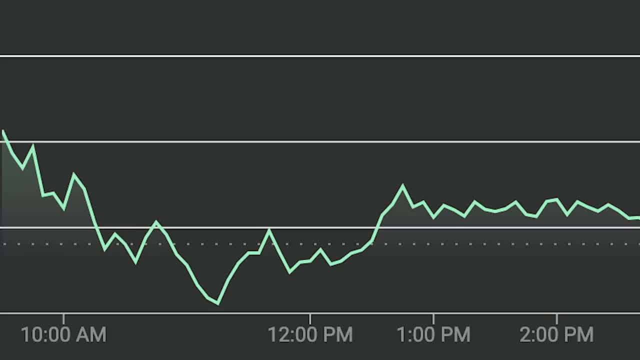 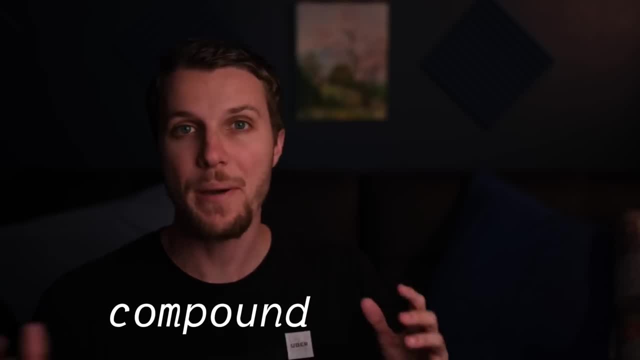 but if we put it together with a bunch of stock prices- let's say the price is over an entire day- well then it becomes more meaningful. We call data items that we group together like this compound data. We have to store this data in some kind of a data structure.